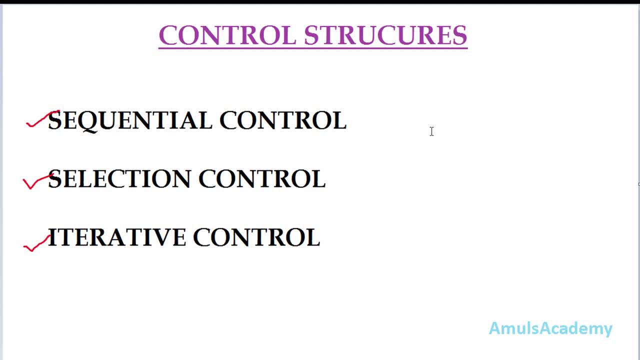 Hello guys and welcome to python programming tutorials by amuls academy. Today in this class we are discussing about control structures. These are the controls which will tell in which order instruction will be executed in our program. For example, imagine that your program contains five lines and this control will tell which line will be executed first. 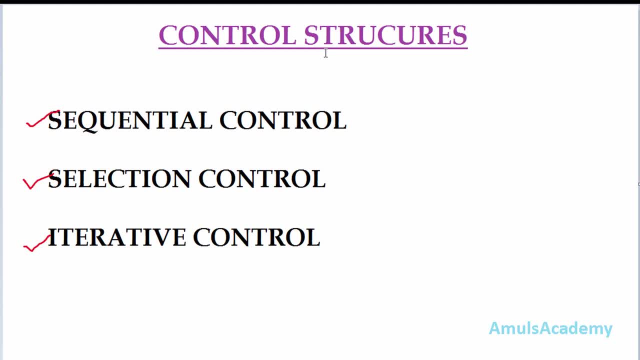 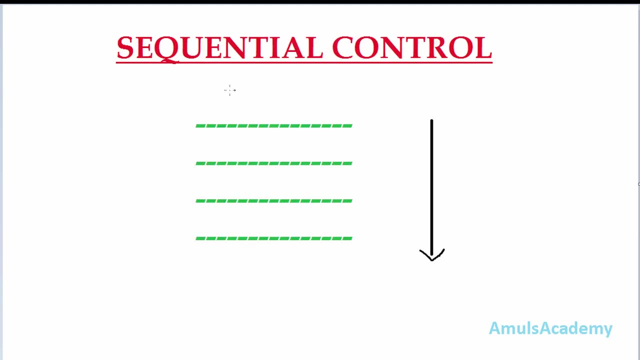 which line will execute next and which line at the last. Ok, there are three types of control. one is sequential control, second one is selection control and the third one is iterative control. We will see one by one in detail. Ok, first we will see about the sequential control. 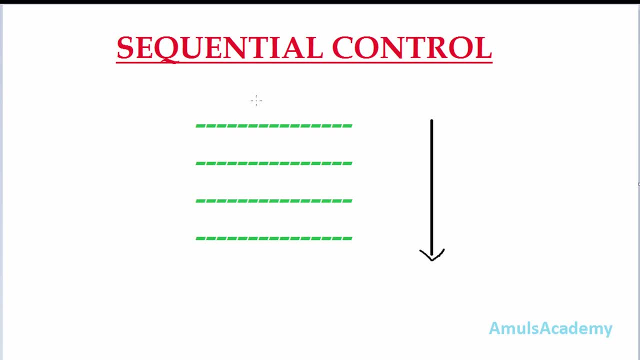 As name indicates, instruction will follow the sequential order. That means it will follow the order in which you wrote your program. That is, first line of your code will be executed first, then followed by second, then third, then fourth. Ok, this is about the sequential control, Ok. second one is selection control In selection. 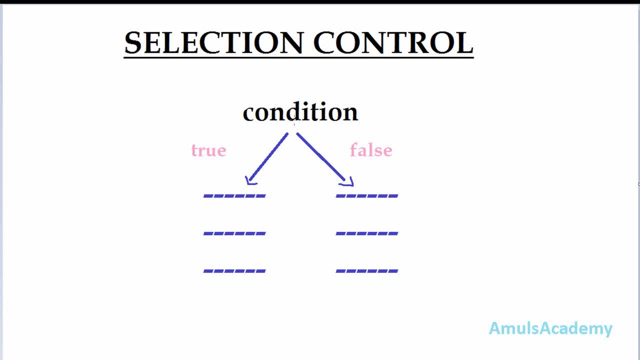 control. there will be one condition. Based on that condition, the statement will be executed. For example, if this condition is true, then this part of the code will be executed. If it is false, then this part of the code will be executed. So there will be a selection. 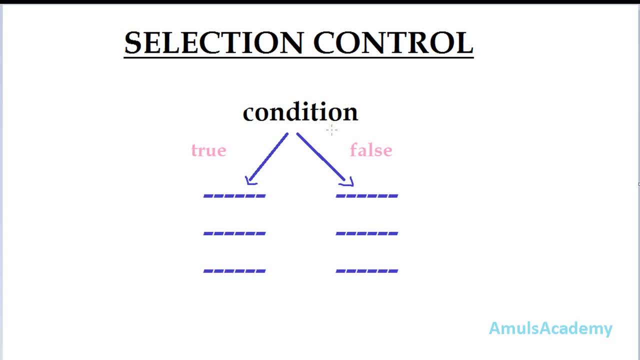 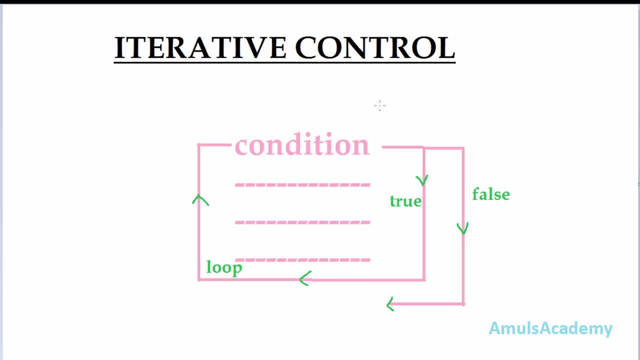 between the statements. so it is called as selection control. This is fully based on the condition. If condition is true, valid, then only this statement will be executed. If it is false, then this statement will be ignored and these statements will be executed. Ok, this is about the selection control. Ok, third one is iterative control. 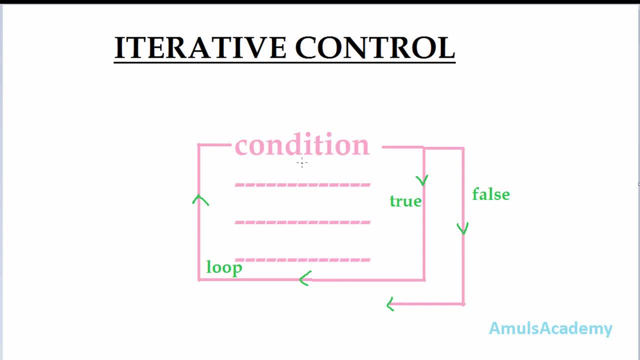 In this case also, there will be a condition. If this condition is true, then this statement will be executed, And again this condition will be checked. If it is again true, then again this statement will be executed. Until the condition become false. this statement will be executed repeatedly. 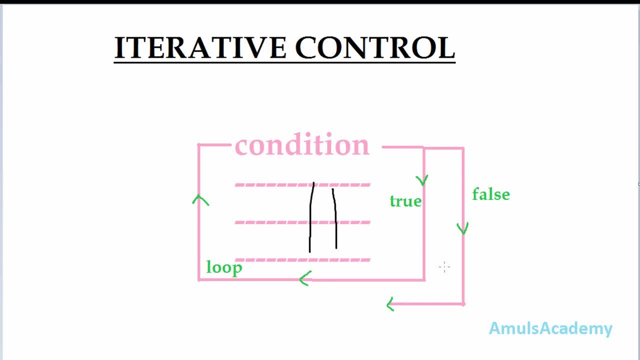 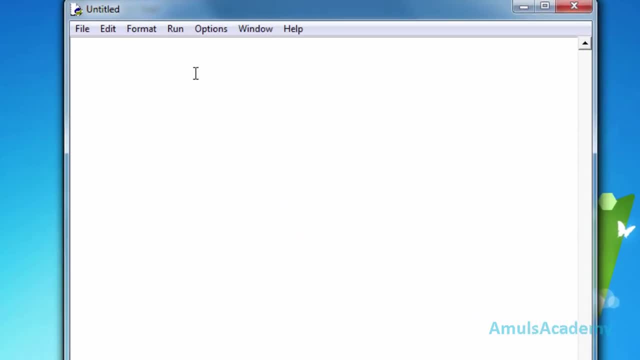 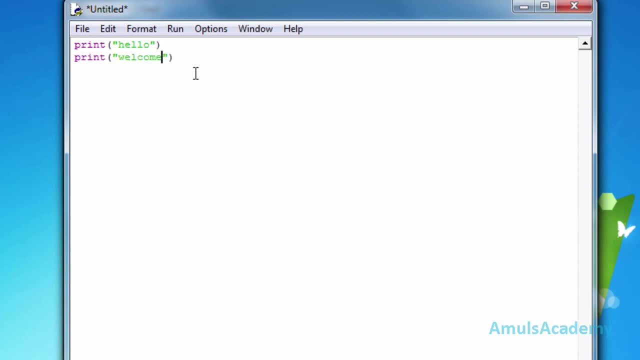 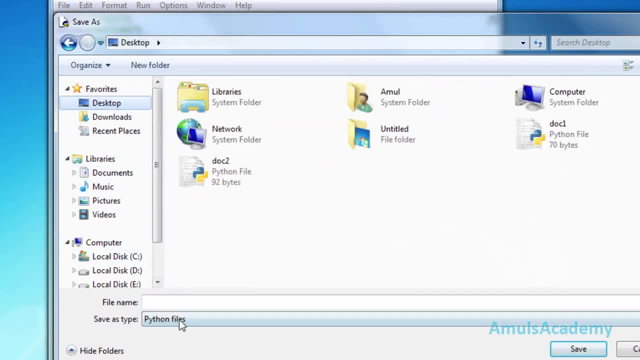 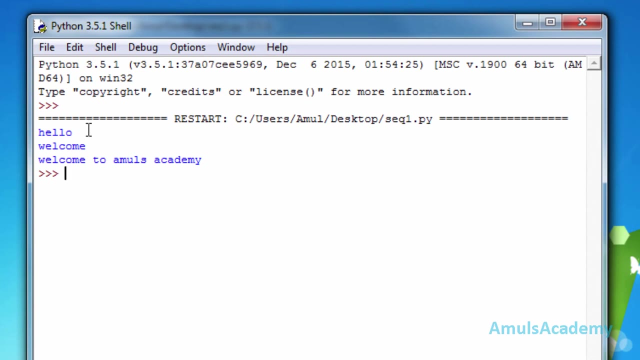 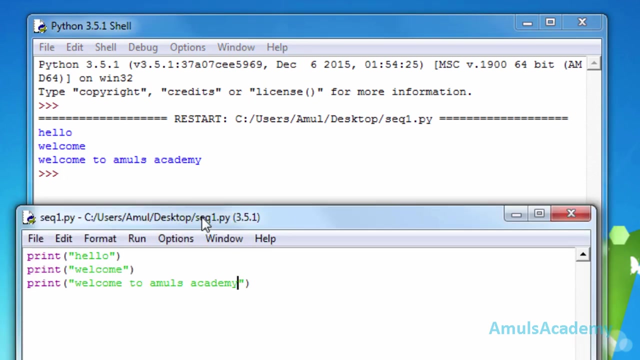 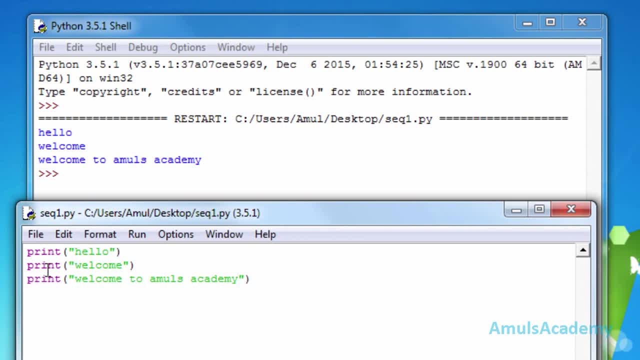 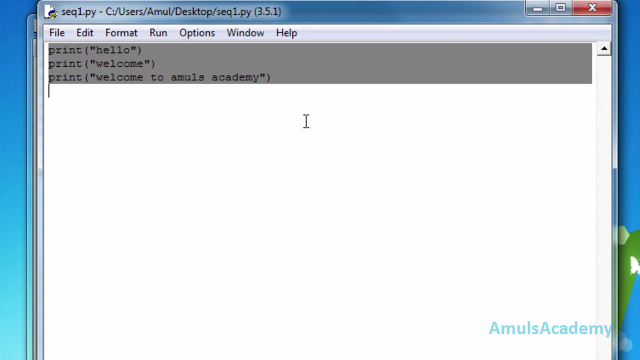 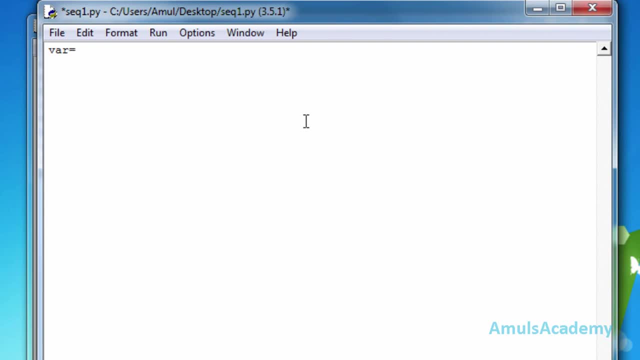 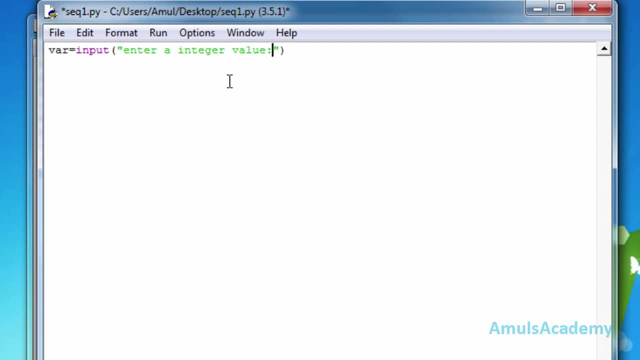 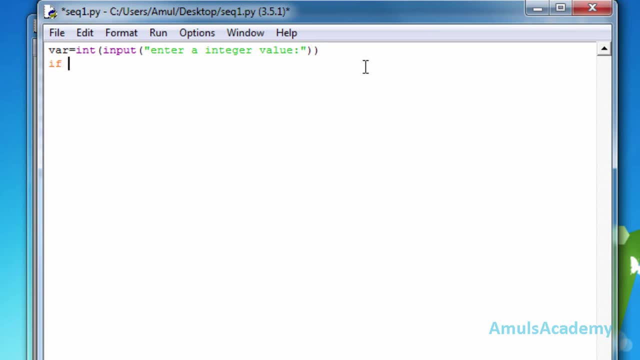 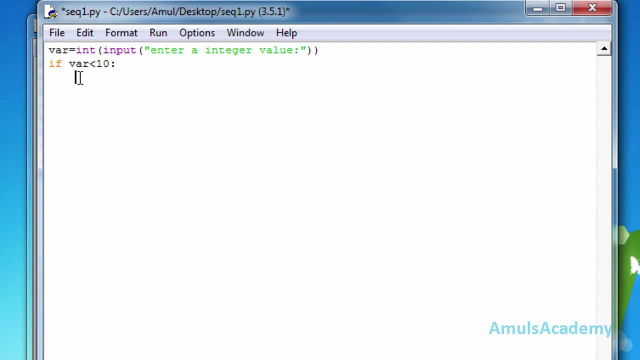 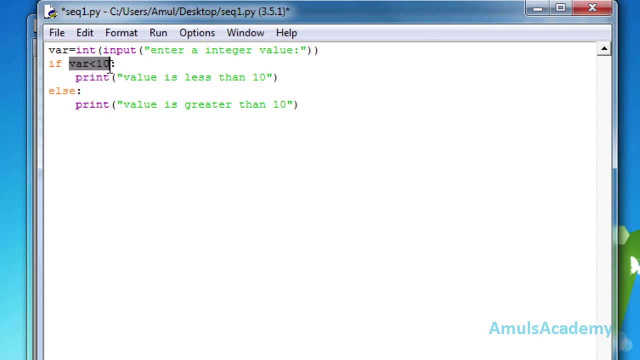 there will be one condition that is variable: less than 10. if this condition will be true, then it will be less than 10.. then it will be less than 10.. then only this statement will be executed, that is, value is less than 10 if condition. 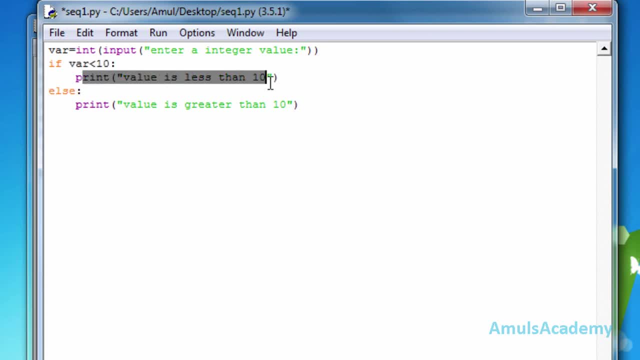 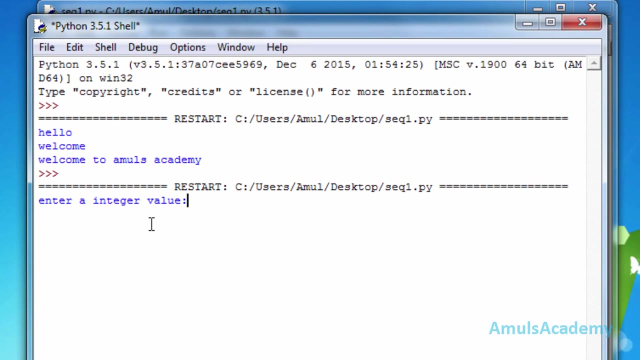 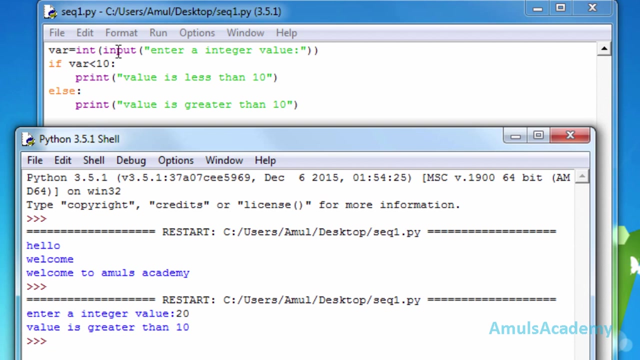 is false, then it will be ignored and else part will be executed. ok, so for this, save this run run model. ok, now we need to enter a integer value. so i will write 20 and i will press enter. here value is greater than 10. here i entered the value 20, so var will hold the value 20. 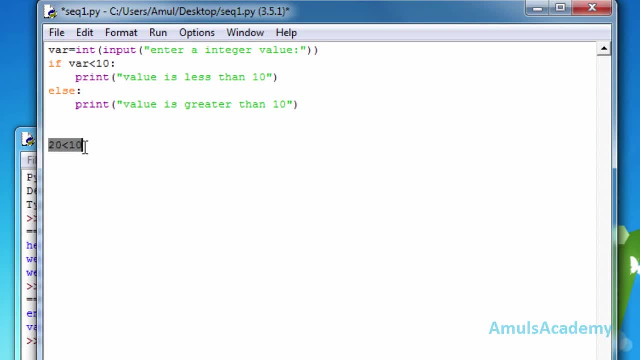 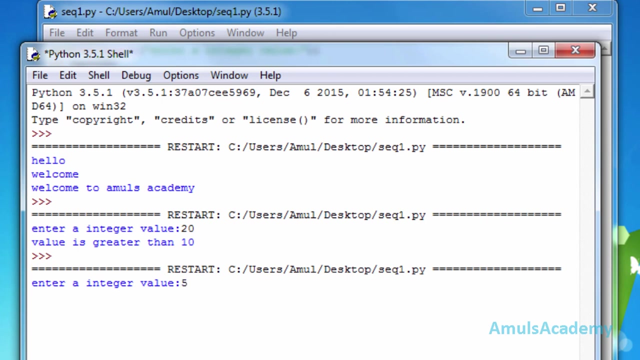 so it will check whether 20 is less than 10. no, it is false. so this statement will be ignored and else part will be executed. so we are getting answer as value is greater than 10. now we will again execute this file. so now i will write the value as 5 and enter. we can see value. 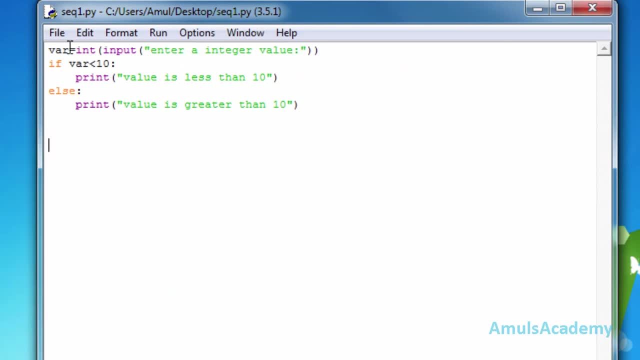 is less than 10, it's because i entered the value 5. 5 is less than 10, so it is true. so this part will be executed and else part will be ignored. here there is a selection of the instruction based on the condition, so it is called as selection control. there are different. 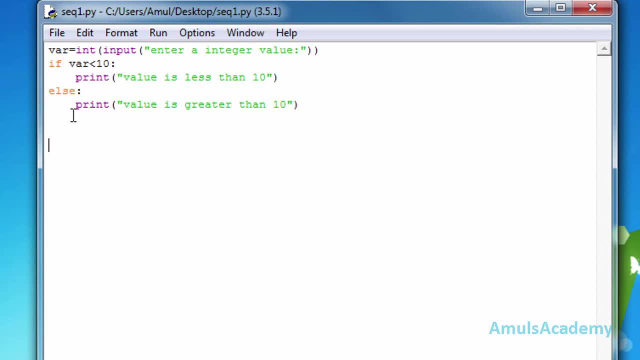 types of selection control. one of them is: if else, i will explain different types of selection control in next class. ok now. third one is iterative control. for that i will create one variable, var. i will assign the value 0. now i will use iterative control. that is while. and here we need to mention: 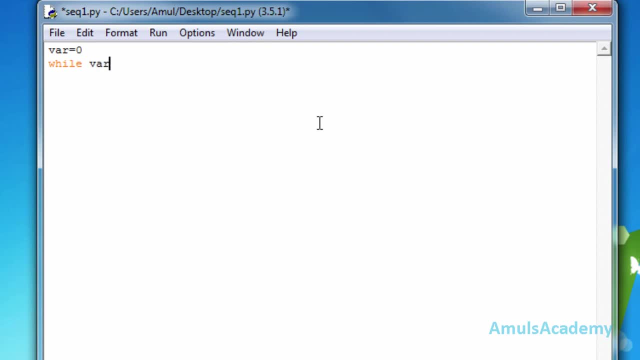 the condition. so i will write var is less than 10.. and colon enter and i will type print and var. next line i will type var equal to var plus 1. this statement is called as increment, while containing three part. one is initialization condition. third one is increment or decrement. ok, 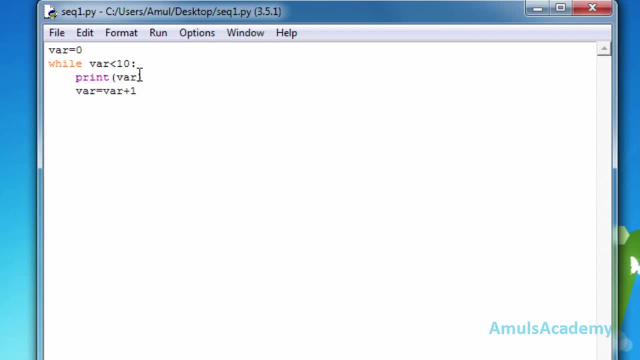 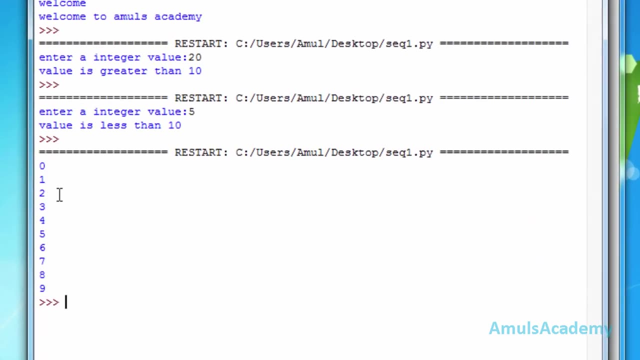 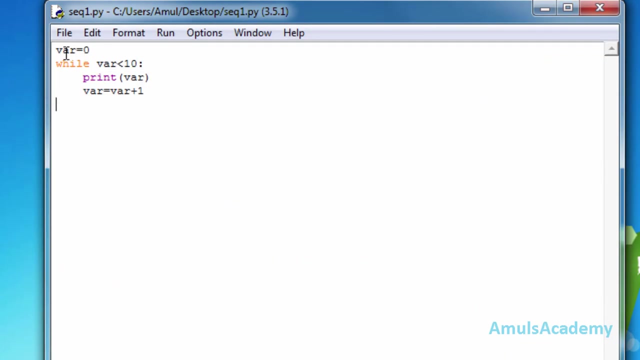 now i will save this file. go to run and run module. we can see the output as 0, 1, 2, 3, 4, 5, 6, 7, 8, 9. why it's because we initialized variable var with 0. now the value of variable is 0. here it will check whether. 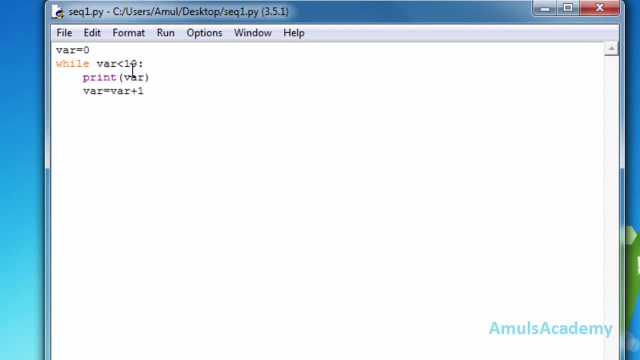 var is less than 10. that is, 0 is less than 10. yes, of course, so it will go for this statement. that is print var. it is for printing the value, so it will print first as 0.. now the next statement is an increment statement. so variable value was 0 here, 0 plus 1 now. 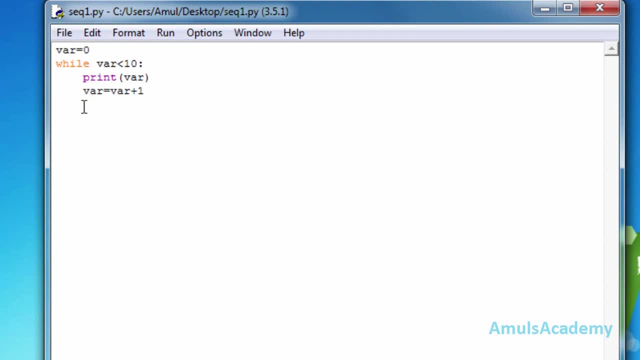 the var is incremented to 1. now again. it will check for the condition. now, var is 1. 1 is less than 10, so value will be printed that is 1.. next it'll come to this statement: actually, var is 1, one plus one. answer is 2. now again.